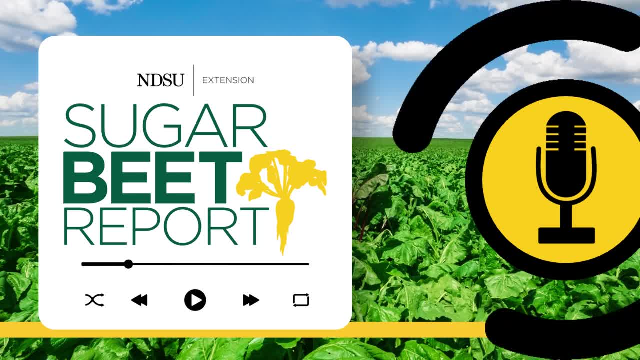 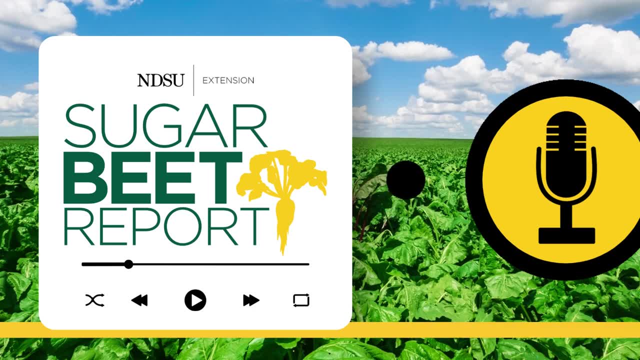 Minnesota Extension Soil Scientist Daniel. market trends have fertilizer prices dropping, so what should producers be thinking about this spring- for current fertilizer applications or for plans for the fall? Well, you know, it kind of depends on where they're at right now. If you've 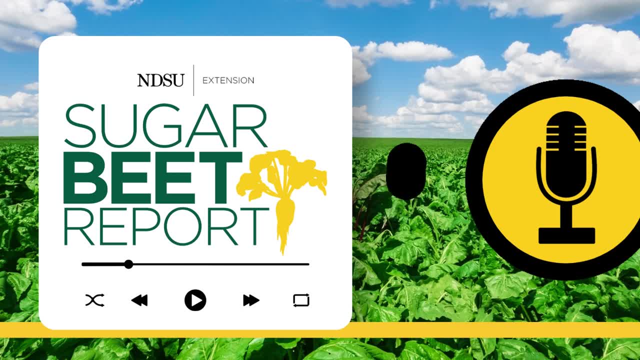 already got decisions made with fall applications. we're kind of missed the boat on things. It is good to see that some of the price is going down, particularly for nitrogen. I don't think it affects sugar beet as much because we don't use price ratios particularly for nitrogen for. 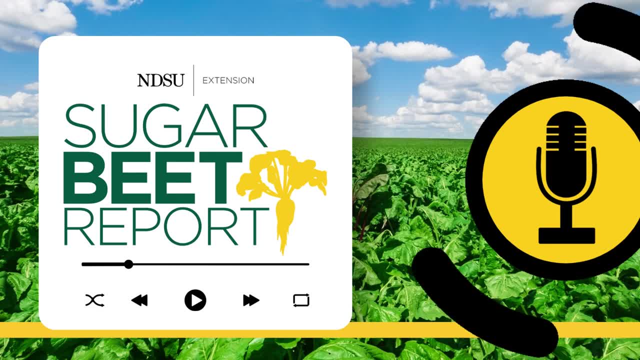 managing the crop. But I think the big question for beet growers will be looking at residual nitrate trends, if you are looking at that, because that's been the biggest question the last couple years with the fall. So I think it's a good idea to look at that. I think it's a good idea to look at. 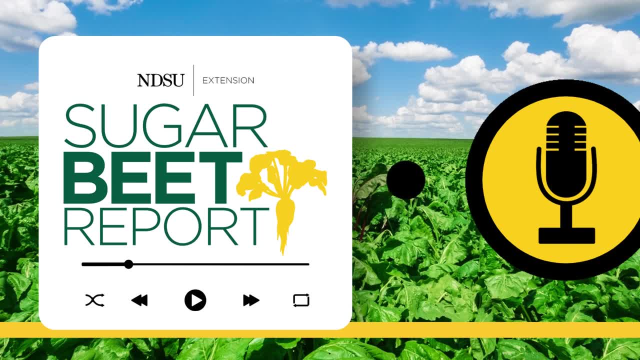 the dry years, how much residual nitrate we're carrying over. Now just looking at some of the data from closer to the southern region and the northern region, from MVTL and AgVice, and the numbers have really been trending down. I was kind of surprised looking at some of the 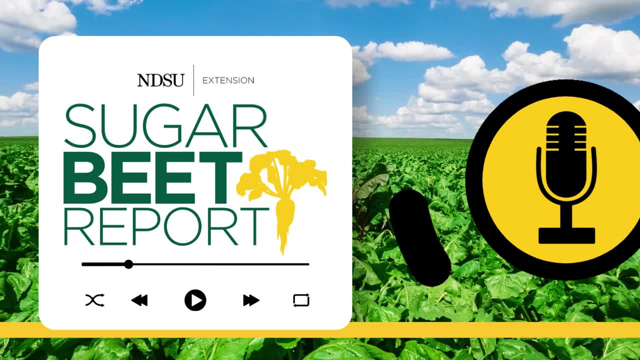 median values, particularly from MVTL. I would expect that a lot of the growers in the southern region, if they're following corn, to have potentially higher residual nitrate just because we tend to see that in the last few years. But that hasn't been the case, I still think. 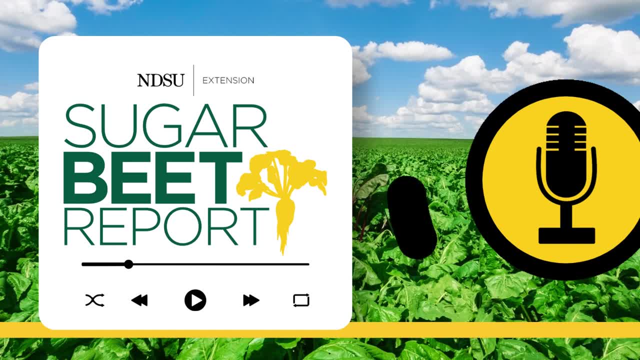 for growers. I would be paying attention to that. For what you have for current guidelines. it hasn't really changed, So I'll be evaluating that, moving forward as I've been collecting more of the data from some of the past researchers working on sugar beet in northern and. 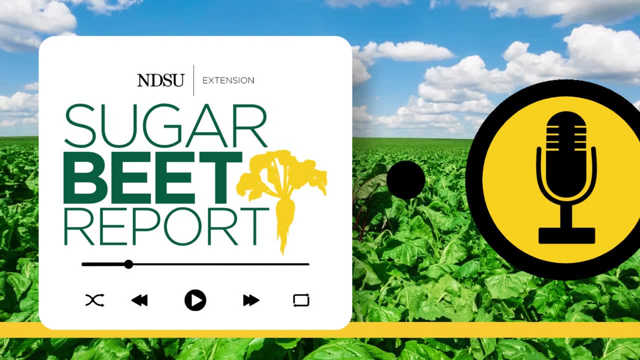 southern Minnesota, But no major changes right now. I think the main thing for fall will be anybody that's been holding off on phosphate and potash applications. If the prices do tend to trend downward, I would just be rechecking some of your soil tests, especially if you've had some fields. 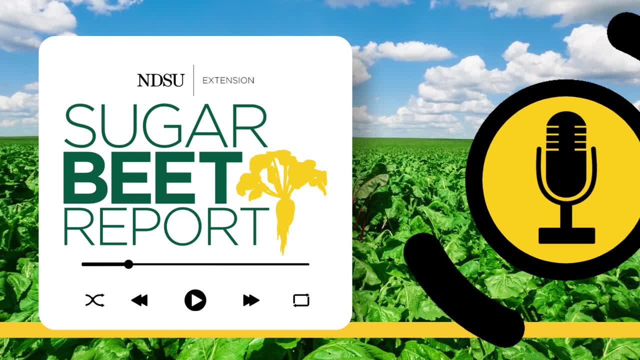 you've gone a little leaner than normal on just to see where things are at, Because I would suspect we'll see things moderating around a 0.1 price ratio. It's kind of what we see: a 0.1 price ratio. 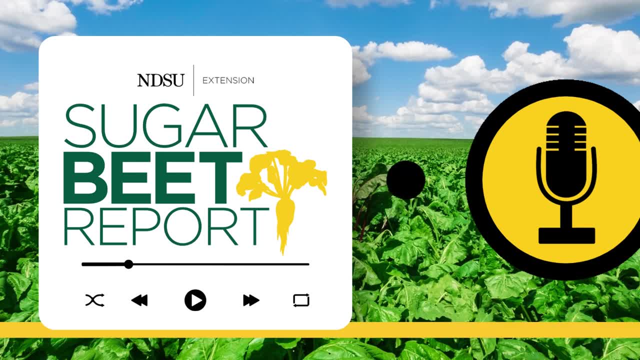 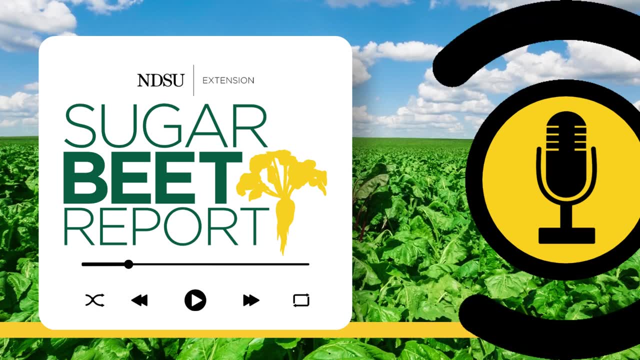 in relation to the corn price for most of our nutrients, And if that's the case, I guess I would just be re-evaluating the soil tests. If you get a chance, maybe going into some fields maybe a little earlier than normal. For beet specifically, I don't think you're going to see any surprises in. 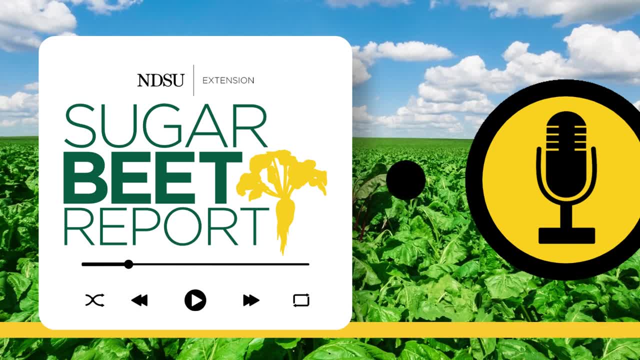 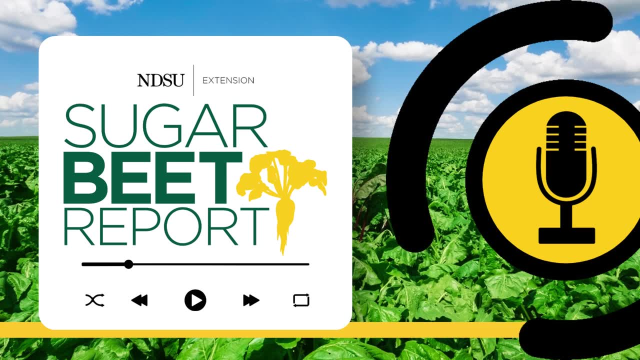 what's in the current production guide. That's kind of what we've been looking at focusing on, But I'll be evaluating that moving forward as I get more geared up with sugar beet research. Outside of nitrogen, phosphorus and potassium, are there any other nutrients that we should look at this spring? 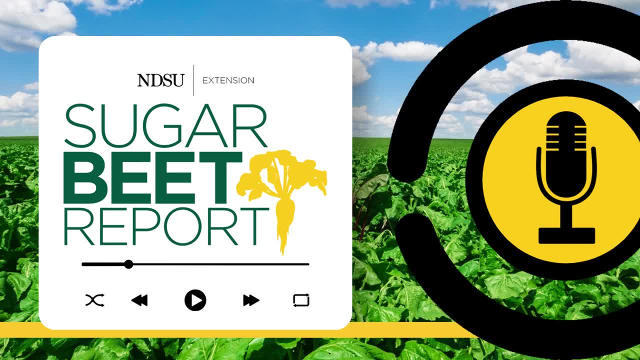 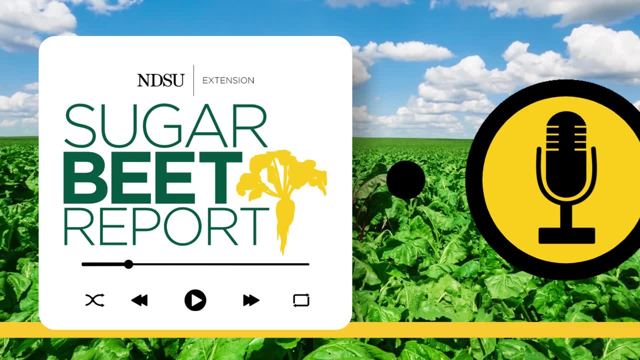 Well, it's going to depend on what we see. Sulfur is always the one that tends to come up more often than not. Last year, going up north around Crookston, when we got some of the crops in late, I was seeing more sulfur deficiencies on corn. I wouldn't expect it with sugar beet- A lot of our. 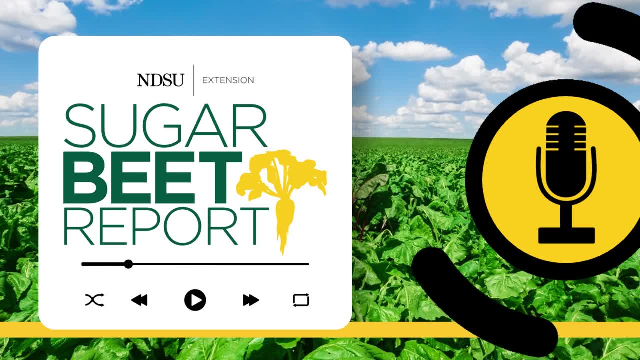 data really doesn't show much of a benefit to sulfur for sugar beet production. In many of those soils, and particularly with a crop that is a deep taproot, you've got a lot of sulfate probably deeper in the profile, which I wouldn't really expect. 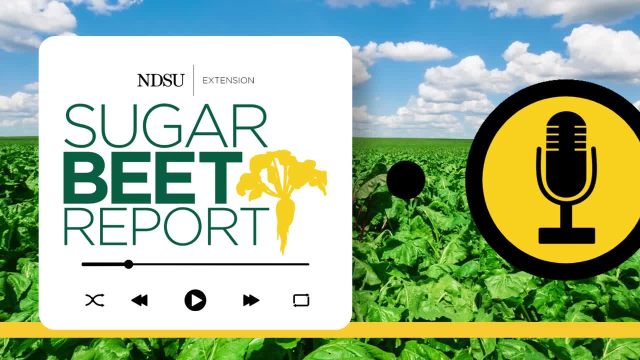 Much of an issue with that nutrient, unless you've got some pretty sandy soils. The other thing that tends to come up more often than not is boron. We did hear some talk- that's been a couple years ago- of some low boron tissue concentrations in some of the sandier soils. 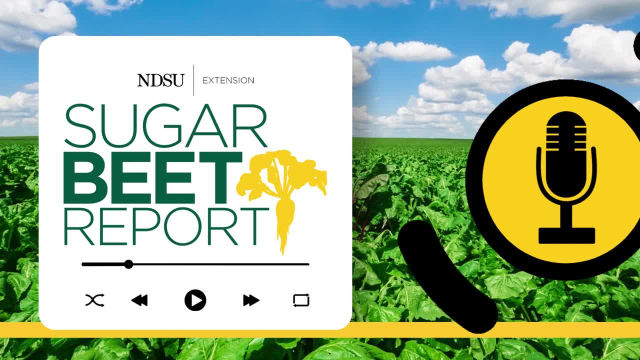 I'm still not recommending widespread applications of micros. I mean boron is one of them. If you do have very sandy soils with low organic matter, I mean certainly you could see some lower tissue concentrations, But I don't know if that's a result of. 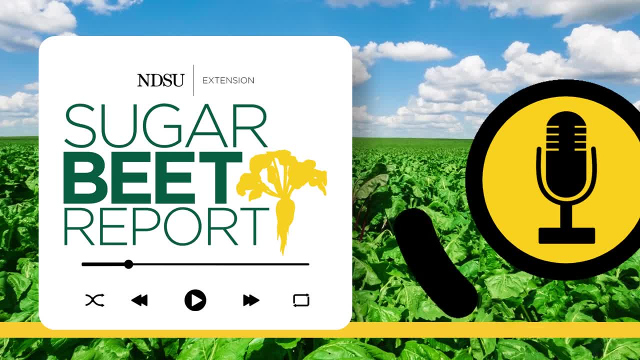 you know, being actually lower, just the dry weather, because we tend to see dry weather and low tissue concentrations come into play. And the other one is manganese. That one does come up as well. You know, looking at a lot of the cercospora treatments, some of them will. 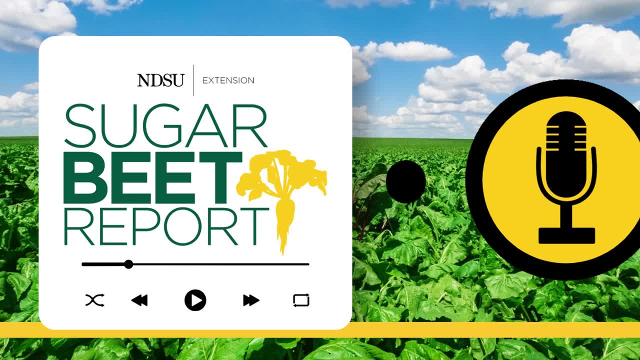 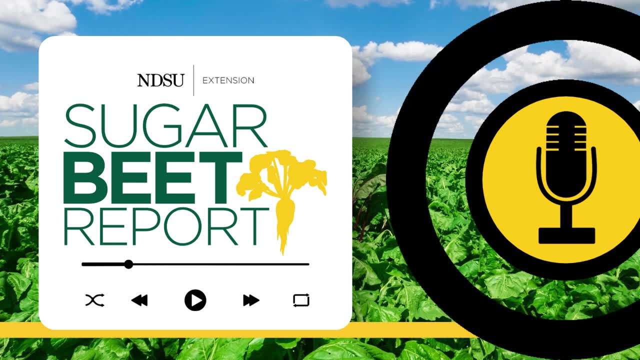 contain manganese applications as a foliar, I just wouldn't really be too concerned about it. I think really, looking at your basics- nitrogen, phosphorus and potassium is really what you're going to want to look at, because it's really where you're going to make the most of your 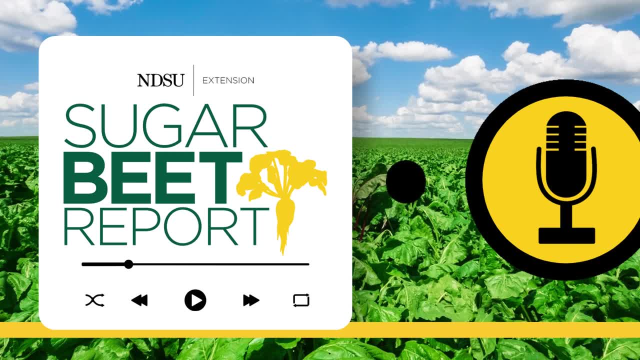 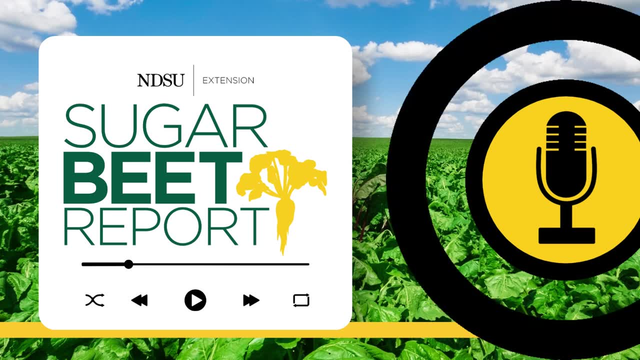 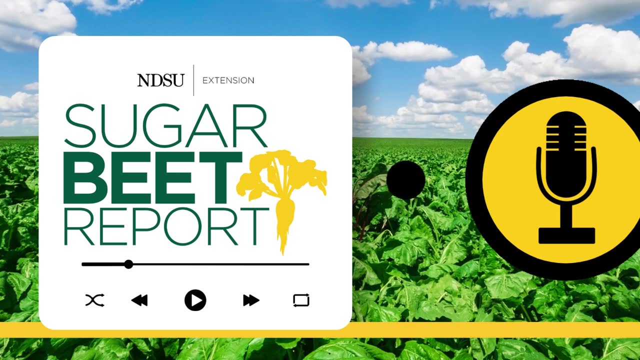 money when it comes to either increases in tonnage recoverable sugar. When we start looking at these other things, it just isn't a high enough chance of return. Are biologicals something that growers should be considering to incorporate into their fertilizer programs? Biologicals are one of those interesting things that you know I'm getting a lot of. 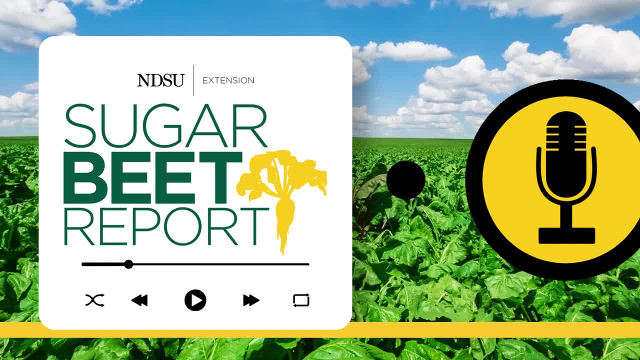 questions on it, but there just isn't a lot of data on specific products. Just looking at, a lot of these are geared towards corn. I mean we start talking about other crops. There's a lot of unknowns. The thing I can say about a lot of these products is inconsistency. Most of the data shows